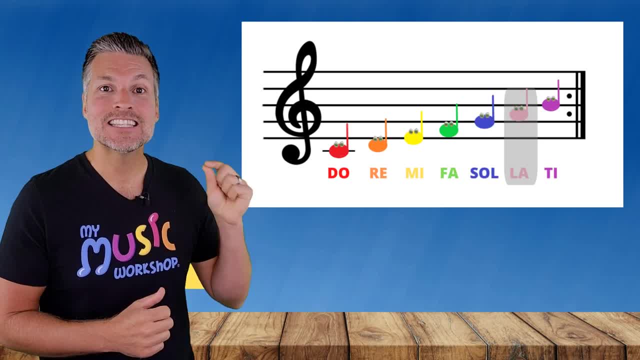 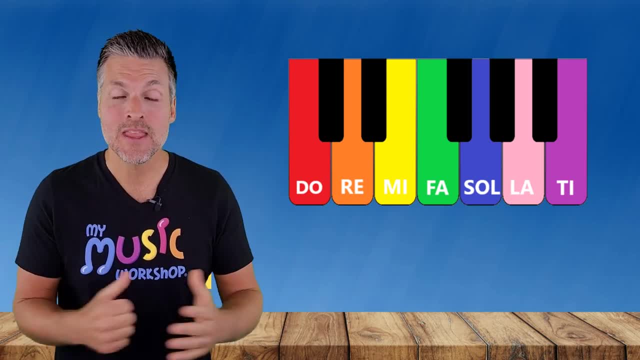 re mi fa sol la ti. Now, each one of those sounds is going to be one of the notes in the scale when we sing. Now you can use solfege for other scales, but right now we're going to use it for the C major scale. 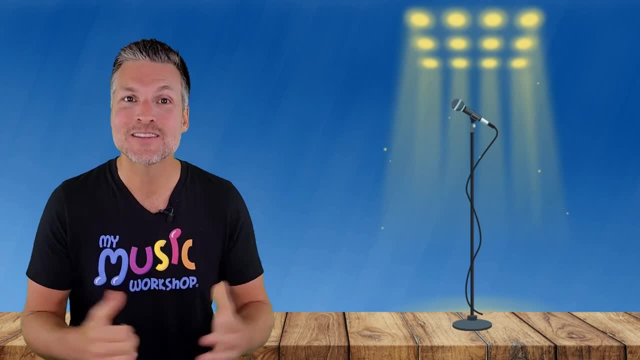 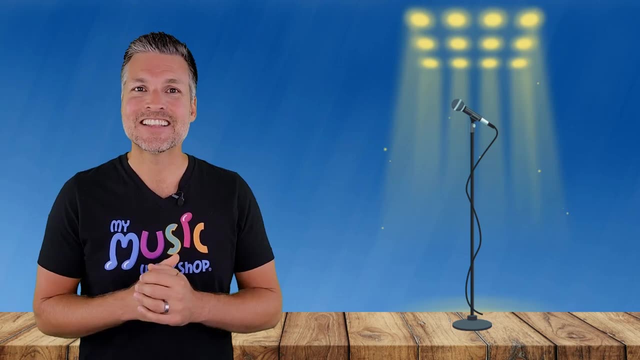 Are you ready to start singing using solfege? I am so excited. You're an amazing singer and we're going to learn some more in the next lesson. Here we go. Hi friends, Are you ready to start singing using the first three sounds in solfege? 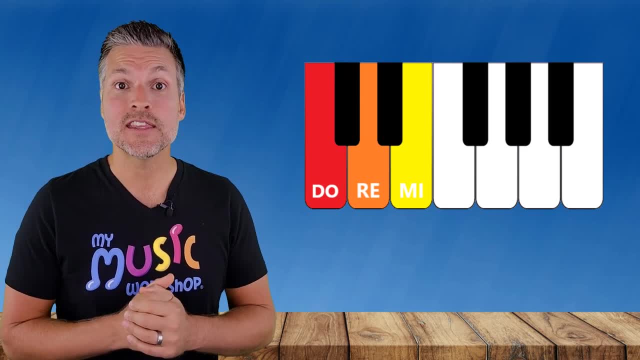 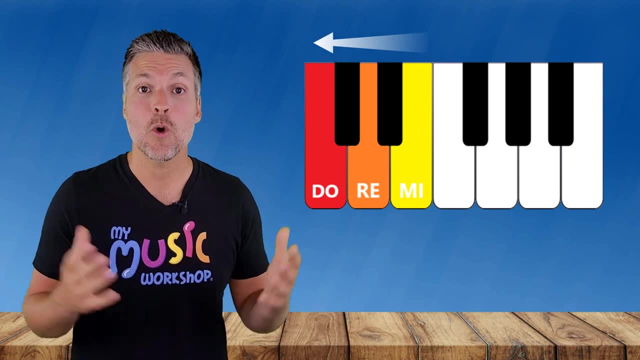 Now those sounds are: do re mi. You're going to listen to what the teacher does and then you're going to sing the same thing. She's going to go up with the sound or higher, and she's going to go down with the sound or lower. 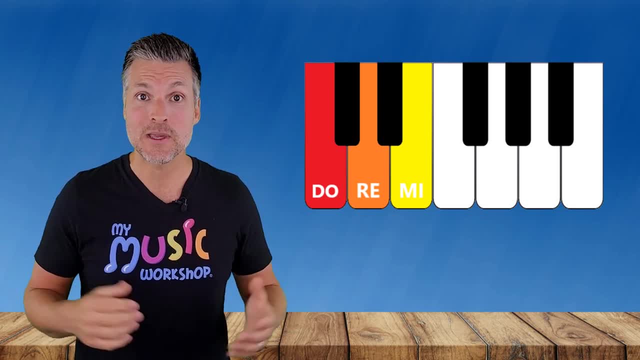 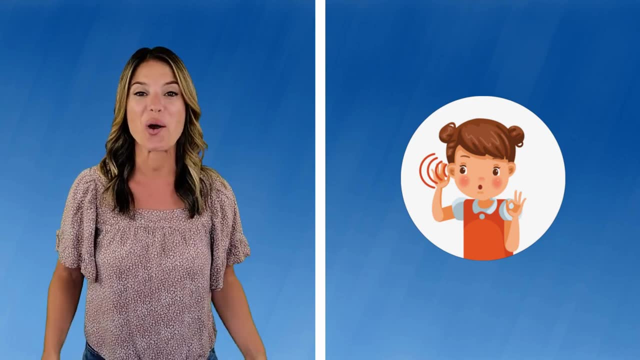 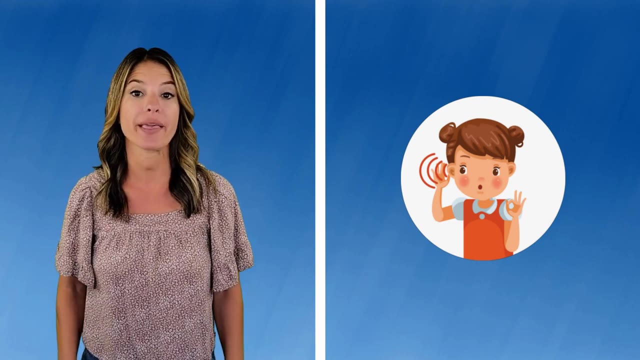 You can do it. I want you to have tons of fun. Here we go. Let's sing: Do re mi, Do re mi, Do re mi, Mi re, do, Do re mi, Do re mi, Do re mi Mi re do. 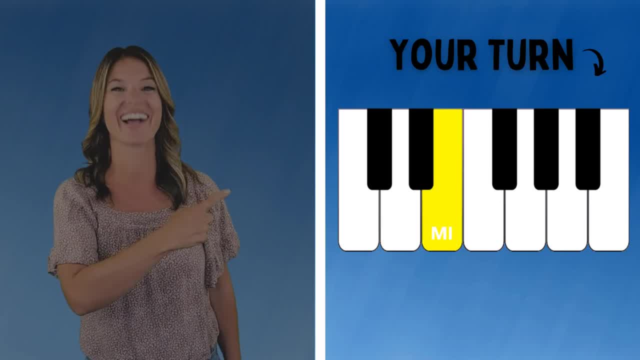 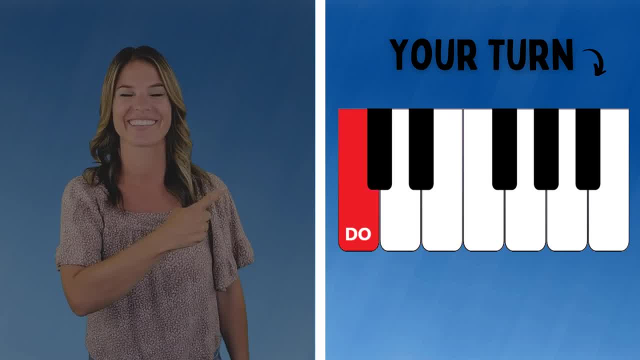 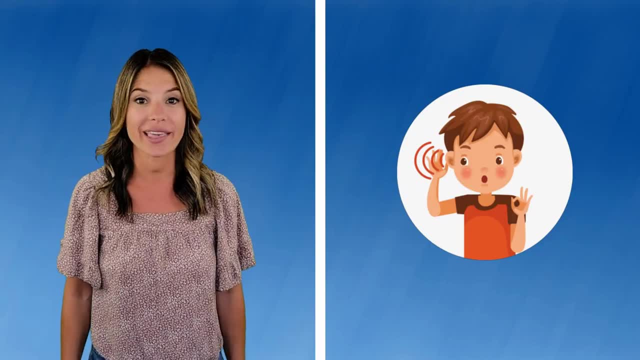 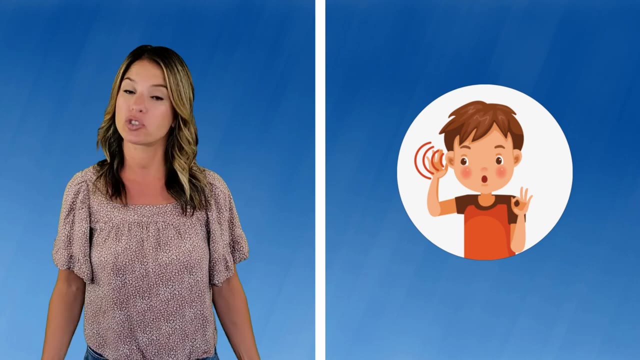 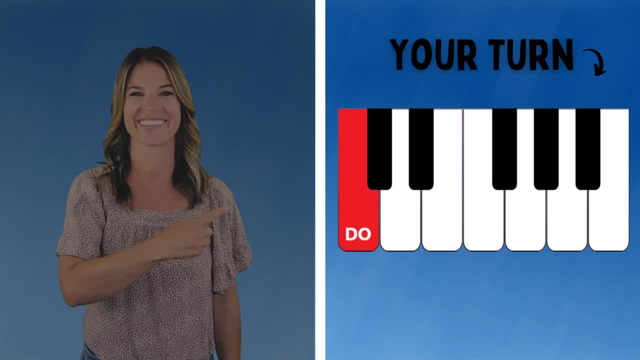 Do re mi, Do re, mi, Do re, mi Mi re, do Do re, mi, Do re mi, Mi re, do, Do re, mi, Do re, mi, Mi re do. 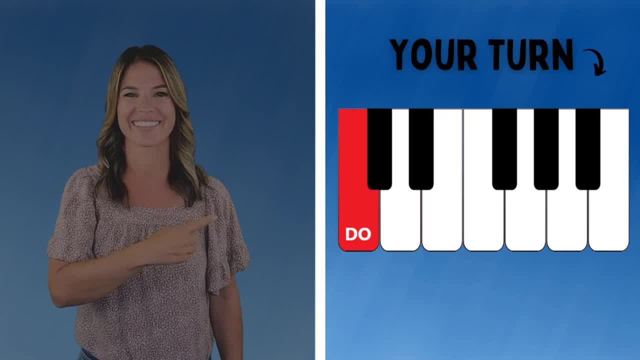 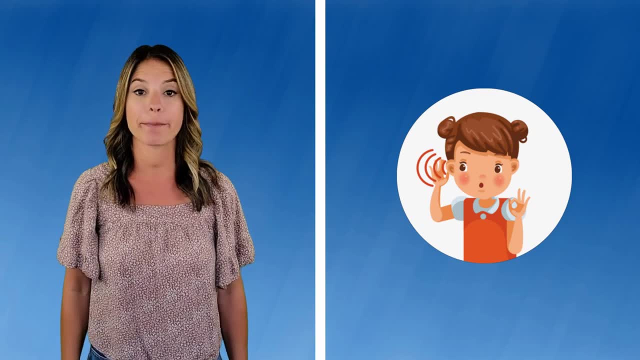 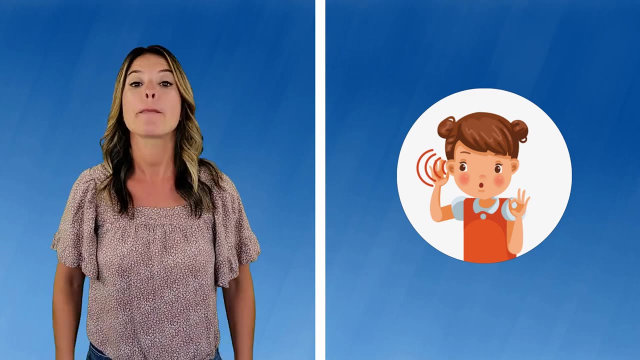 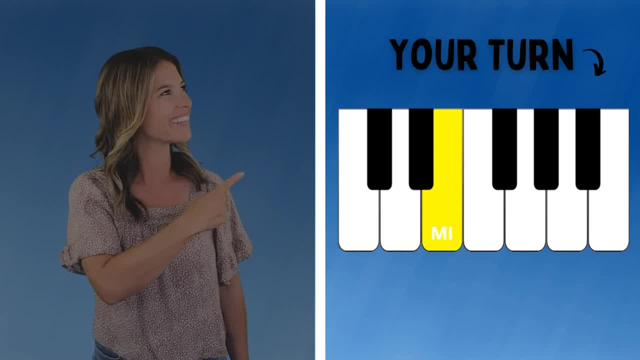